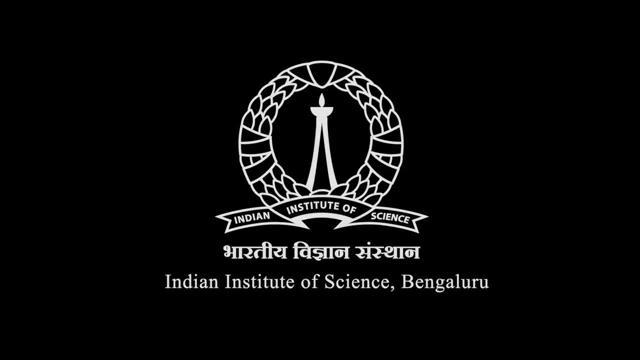 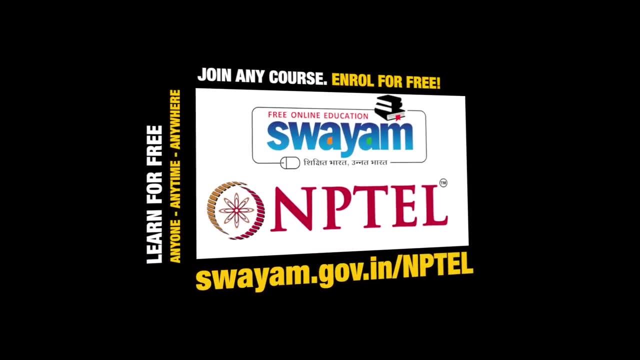 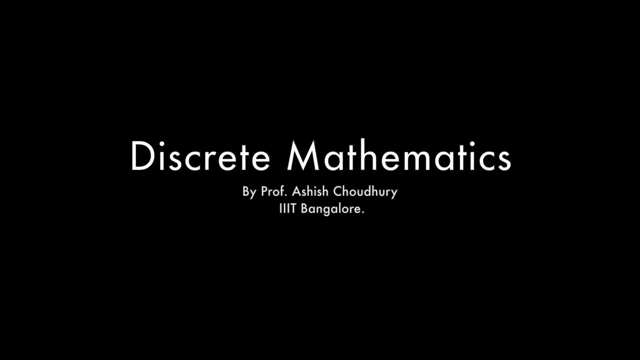 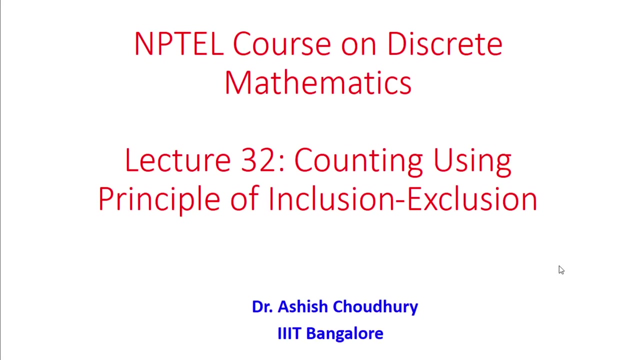 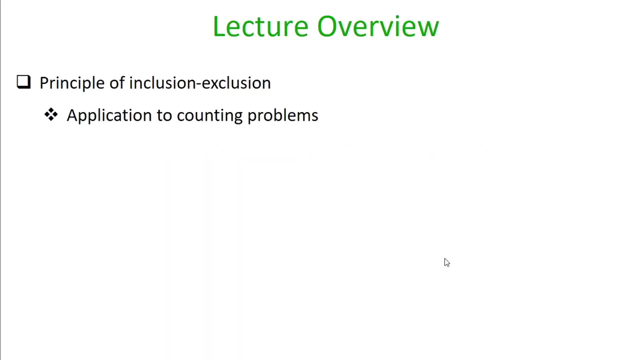 So hello everyone, Welcome to this lecture. The plan for this lecture is as follows. In this lecture we will introduce the principle of inclusion-exclusion and we will see some of its applications to various counting problems. So what exactly is the principle of inclusion-exclusion? 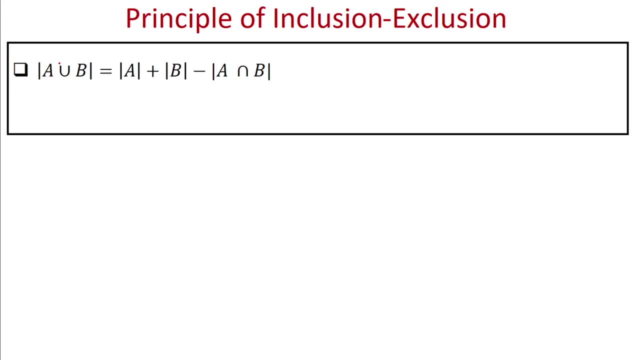 Well, it basically says that if you want to find out the cardinality of the union of two sets, then it is same as taking the summation of cardinalities of the individual sets and subtracting the cardinality of the intersection of the two sets. And why this is true? Because 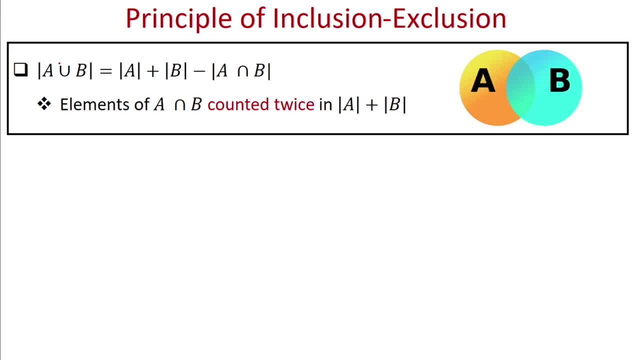 if we see pictorially, or if we follow the Venn diagram method, then if we just add up the cardinalities of the A set and B set, then the common portion or the elements which are common to both sets A and B are counted twice. So to compensate, so so, so so to 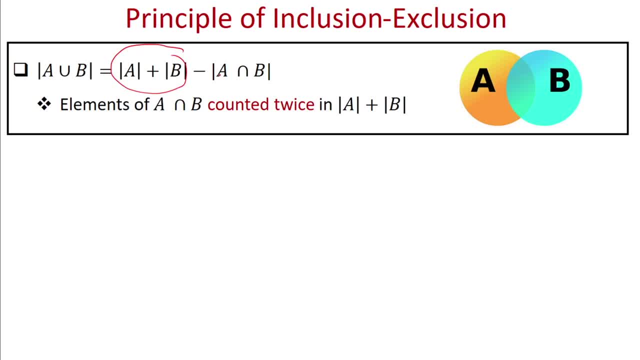 avoid this overcounting. we basically subtract the cardinality of the intersection of the A set and the B set, Now extending this principle to the case of three sets. if we want to find out the cardinality of the union of three sets, then it is the summation of the cardinalities. 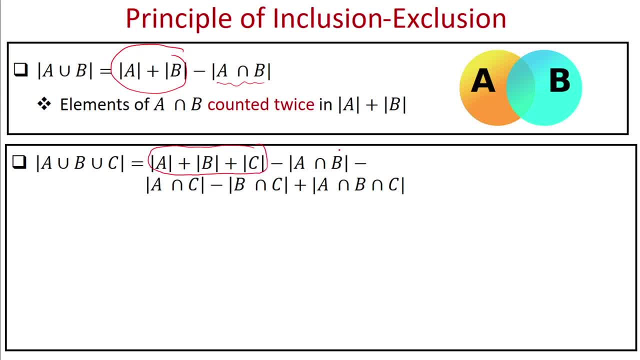 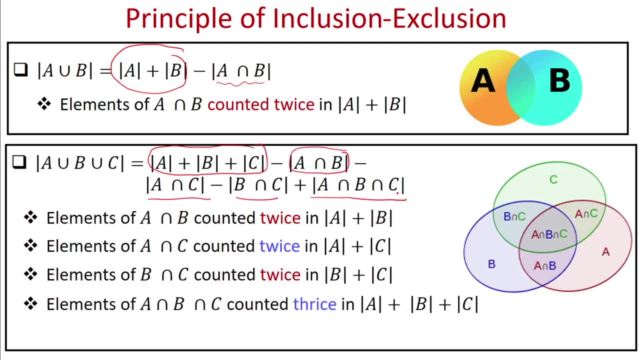 of the individual sets. Then we have to take the difference of the cardinalities of two sets at a time. Then again we have to add the cardinality of the intersection of all the three sets. Again, we can prove it easily using the Venn diagram method. So why we are subtracting? 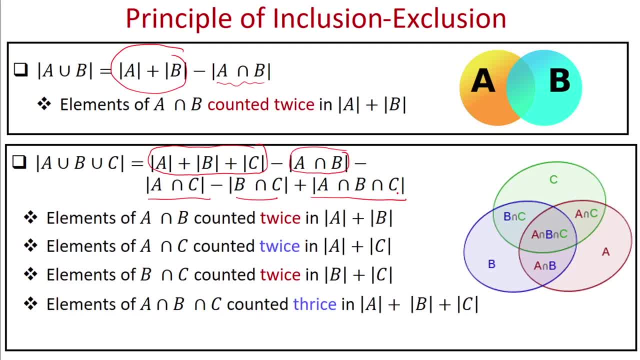 the cardinality of A intersection B, A intersection C and B intersection C, Because the elements in A intersection B are counted twice If we add individually the cardinality of A set and B set. Similarly, when we are adding up the cardinalities of A set and C set, the common portion or 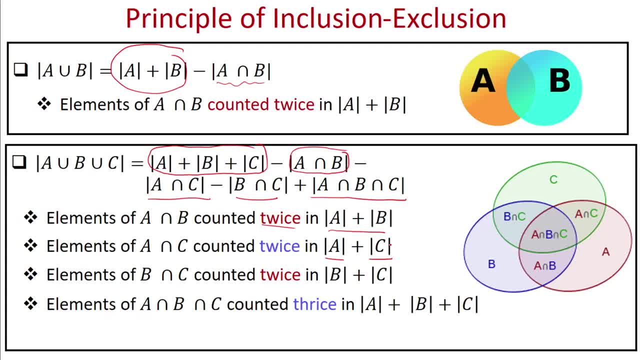 the elements common to A and C are included twice and so on, Whereas the elements which are common to all the three sets they are counted thrice. If we just add up the cardinality of A, B and C, And if we don't add this cardinality of A, B and C, then we have to subtract the cardinality. 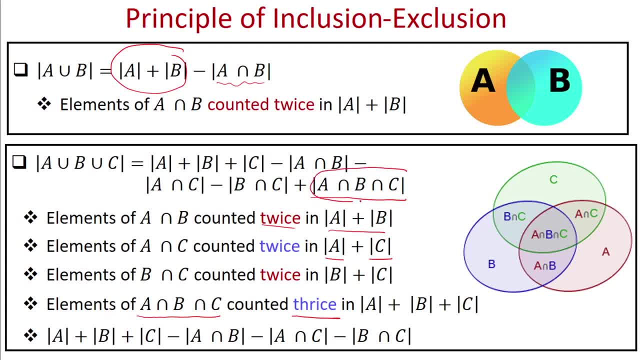 of intersection of A, B and C set and this overall formula Then, because since we are subtracting out the common portion between A and B, common portion between A and C and common portion between B and C, their cardinality, If we don't do this extra addition, then 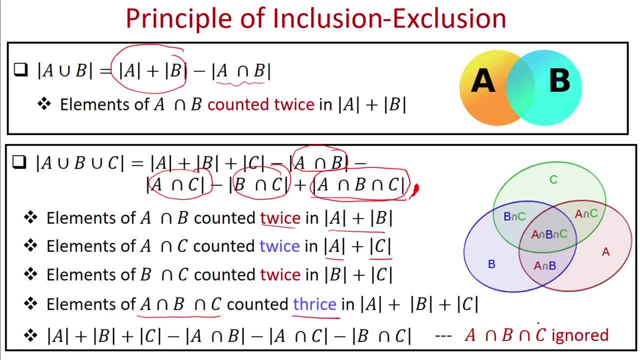 the contribution of the common elements in the cardinality of A, B and C set will be 3 sets- is ignored, So that's why this plus is still. Now we have seen the principle of inclusion exclusion for this case of two sets for the 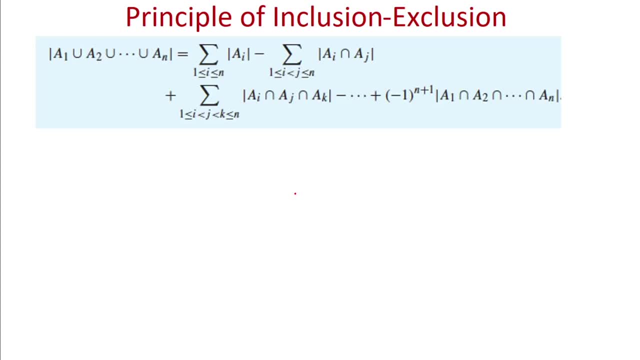 case of three sets, We can generalize it to the case of n sets, right? So the general formula says the following: If you have n sets, they may be disjoint, They may there might be overlaps and so on. Then the formula says that if you want to find out the cardinality, 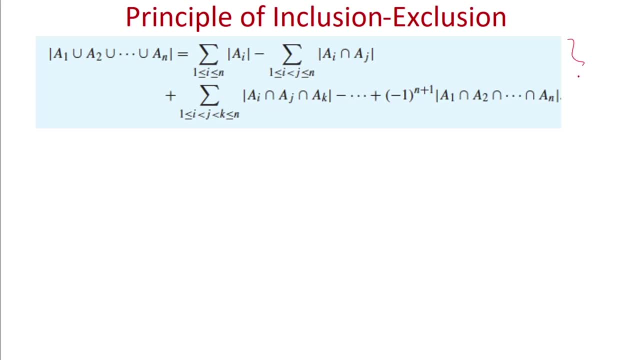 of the union of n sets, then this is this formula. That means it says that it is same, as you have to first individually take the summation of the cardinalities of the individual sets, Then you have to subtract the cardinality of pairwise intersection of sets, Then you 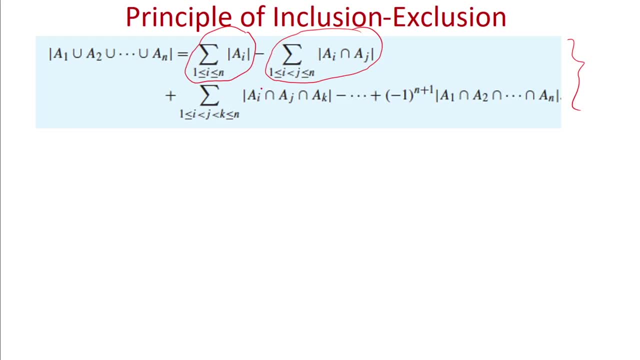 have to add the cardinality of intersection of triplets of sets and so on. That means immediately we alternate: first we add, then we subtract, then we add, then we subtract, and so on. So we have to prove that this formula is correct. You can use proof by induction. 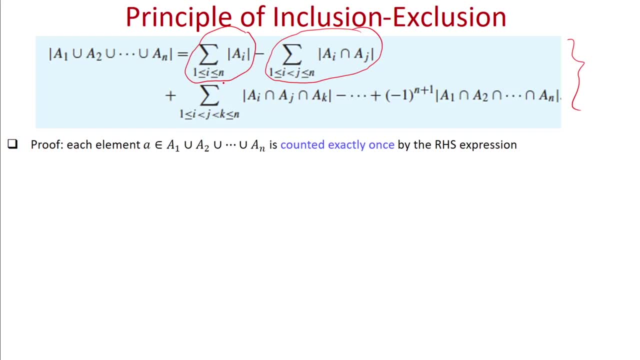 but even without using proof, by induction over n, we can prove it. Okay. So the idea here will be the following: So consider an element, small a, which is present in the union of the n sets. Okay, It might be present in just one of the sets. 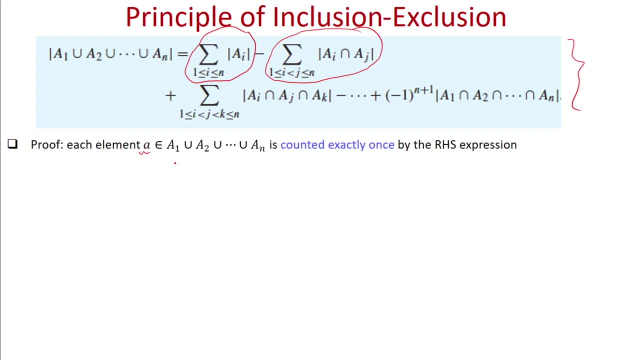 It might be present in two of the sets. We don't know in how many sets the element a is present. We have to show that if at all an element small a is present in the union of n sets, then by this complex looking argument, complex looking formula in the right hand. 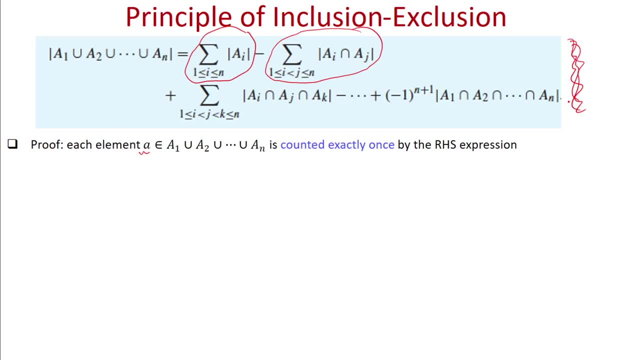 side expression, the element a is counted exactly once, And that's what we want to prove here, basically. So imagine that the element a is present in arg. Okay, The number of sets out of the n sets, where r is at least one, because we are considering 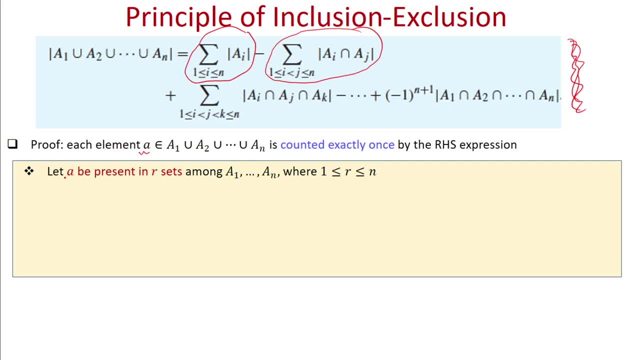 the case where element a is present in the union of all the n sets. So if it is present in the union of all n sets, it's possible only when it is present in at least one of the n sets. And it might be the case that it is present in all the n sets, So that's. 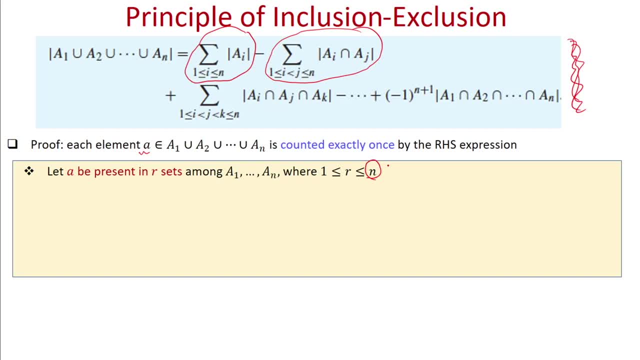 the value of r is in the range one to n. Okay, Now what we have to show is our goal is to show that by the right RHS expression the element a is counted exactly once overall. So for that we observe that the first part of the formula on the right 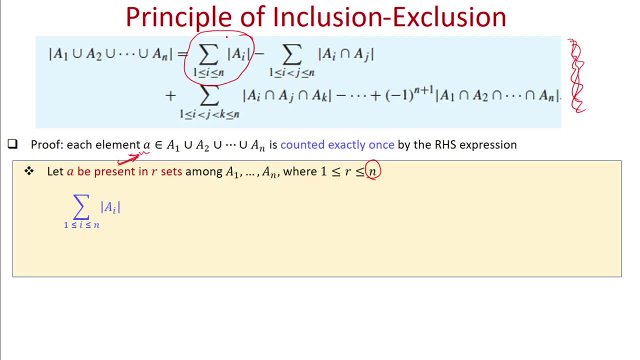 hand side is where we are taking the summation of the cardinalities of the individual sets a1 to a1.. Now, because of this, the element a will be counted R. choose one number of types, right. So, for instance, if the element, if the element, 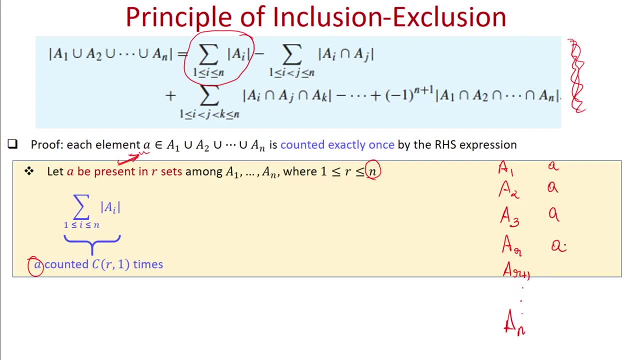 small a is present, say in the first r sets, then because when we are taking the cardinality of a1, the element a is counted once. When we are taking the cardinality of a2, the element a is again counted once. When we are taking the cardinality of a3, the element a is again. 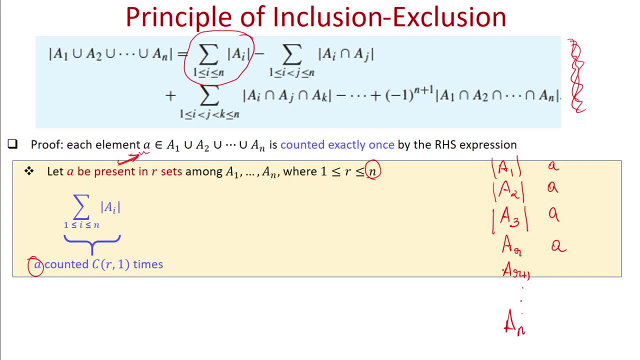 counted once and so on. right. When we are taking the cardinality of a, of r plus one, we are not increasing the count of the element small, a right. So that means through the first part of the formula in my right hand side expression, the element a is counted. 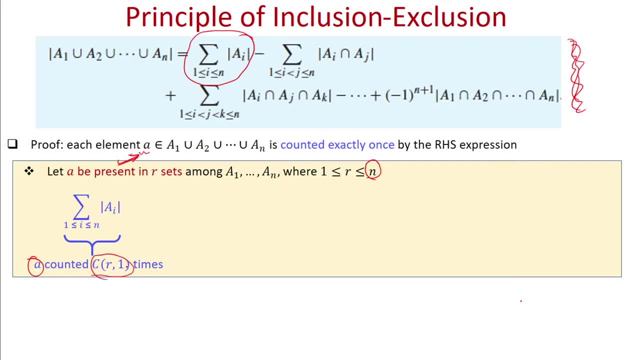 these many number of times. right, Now let's take the cardinality of a3, the element a is again counted once and so on. Now let's take the second part of the formula, where we are taking the cardinality of intersection of two sets at a time, right, So, basically, so it's like saying the following: We are: 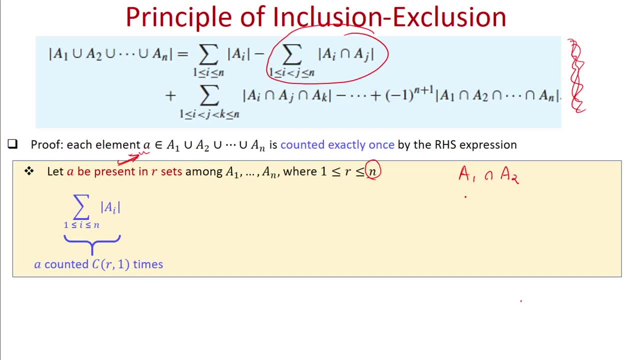 taking the cardinality of a1 intersection a2, a1 intersection a3, and like that, a1 intersection an, and then we are taking the cardinality of a2 intersection a3, a2 intersection a4, a4 and so on, right by the second formula. so we have to find out and when we are taking the. 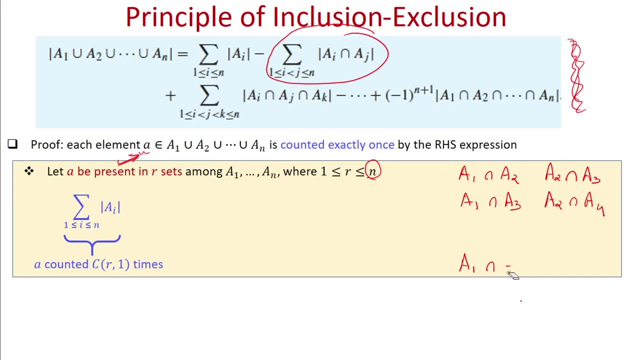 cardinalities of this pairwise intersection of sets, how many times the element a is getting counted. okay, for the moment we are forgetting about this minus here. we are just trying to find out what will be the effect, or how many times the element small a will be counted when we are taking 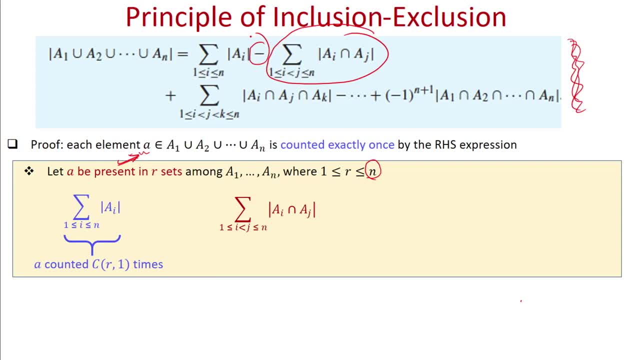 the cardinality when we are taking the cardinality of intersection of two sets at a time. okay, so as per our assumption, the element small a is present in r number of sets. when we are taking the intersection of two sets at a time, element a will be counted only when both the sets where. 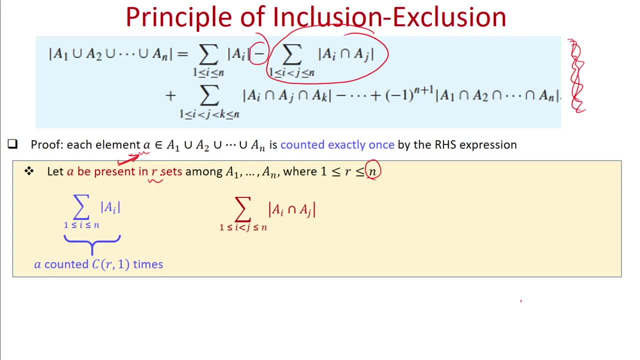 we are taking the whose intersection we are taking, element a is present. if we are taking intersection of two sets where in one of the sets element is small, a is not present, then the cardinality of intersection of two sets will be counted only when both the sets 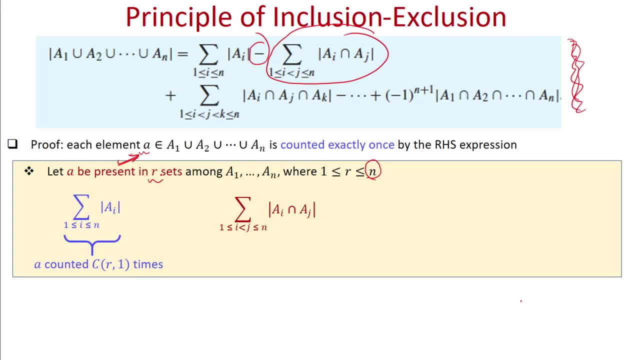 the overall contribution or the cardinality of intersection of those two sets for the count of a small a will be 0, right. So because of this, overall, I can say that, because of the second part of the expression, the element is small, a is counted. r. choose 2 number of times. 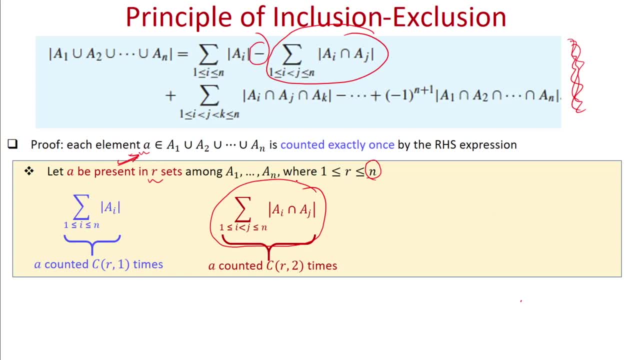 In the similar way, then I can say that when we are taking the cardinality of intersection of three sets at a time, then element a will be counted only when the three sets whose intersection we are taking, all of them, has the element is small a. If element is small a is not present in any, even in one of them, then it would not be present. 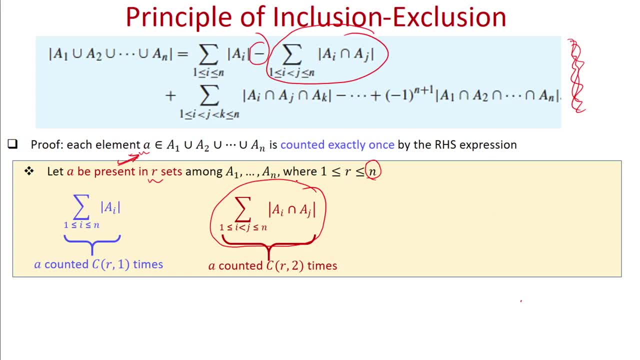 in the intersection of three sets. Due to that, because of the, Because of, Because of considering the cardinality of intersection of three sets at a time, the element a will be counted r, choose 3 number of times And then, if we continue this argument, we can say that when we are taking the cardinality, 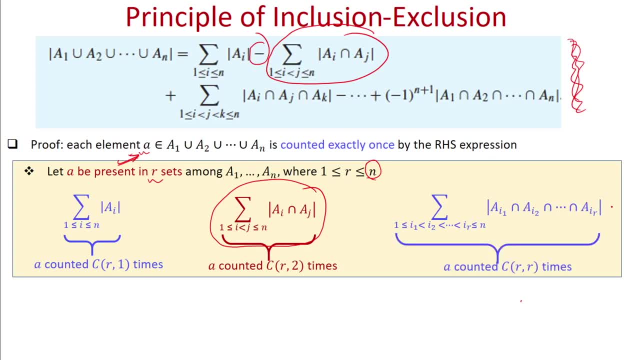 of intersection of r sets at a time, the element small a will be counted exactly once, namely r choose r, number of times and after that, when we are taking the cardinality of intersection of r plus 1 sets at a time, r plus 2 sets at a time, through those parts of my RHS formula, 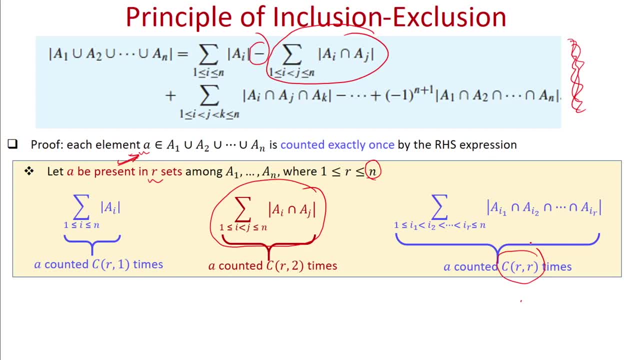 the element a won't be counted at all because, as per our assumption, the element is small. a is present only in r number of sets. So now what we can say is that the total count of this element is small. a by the RHS expression is the following: 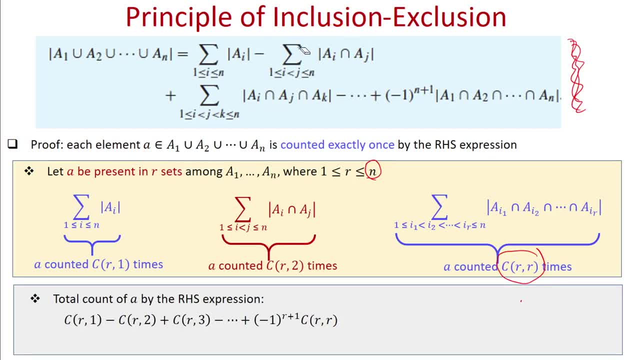 Right. So So, So, So, So So. this is because through the first part of the expression, the element a is counted r choose 1 number of times. Through the second part of my experiment, the element a, the count of element a, gets decremented. 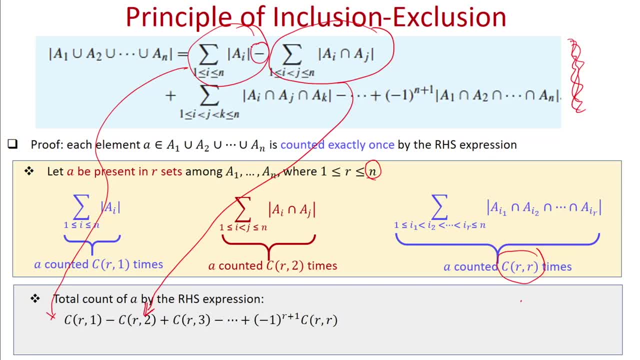 by r, choose 2 number of times. Why decremented? Because of this minus, then due to the third part of the expression, So, So, So, So So, the count of element small a gets incremented by r. choose 3 number of times, and so on, right. 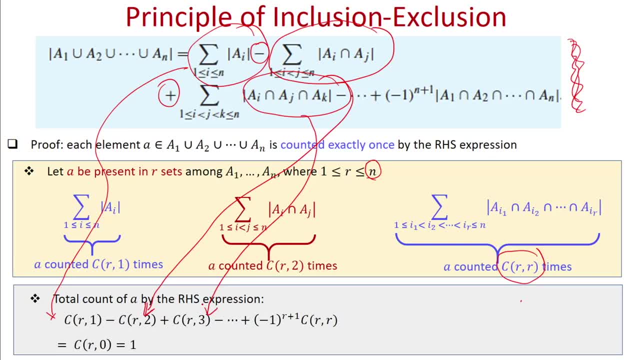 And we know that this expression is nothing but r choose 0. This follows from the properties of the combinatorics function or the binomial coefficients, So it turns out that the summation is same as r choose 0, and r choose 0 is nothing but 1.. 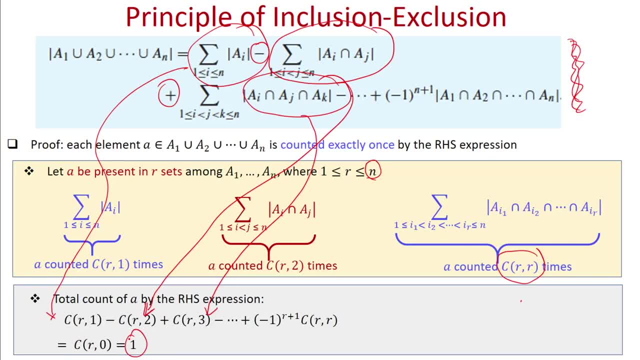 So that shows that by the expression in your right-hand side the element small a, which is present in the union of n sets, is counted exactly once. If there is an element which is not at all there in the union of n sets, it won't be counted at all by the formula right. 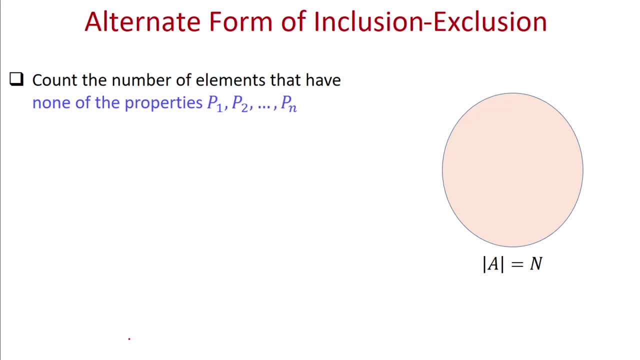 Now what we will do is we will look into an alternate form of inclusion-exclusion which is very powerful, And it is this alternate form of inclusion-exclusion which we use in varieties of problems. So what happens in this alternate form is that we will be facing scenarios where we want to count the number of elements from a set A which has n number of elements, and we will be interested to count the number of elements in this set which has none of the properties, say, p1, p2, p- of n. 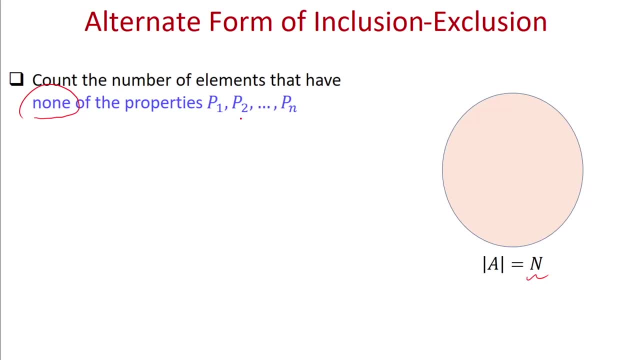 So p1,, p2, pn will be some abstract properties, And we will be interested to find out the number of elements in the set A which neither have the property p1 and nor the property p2,, nor the property p3, and so on. 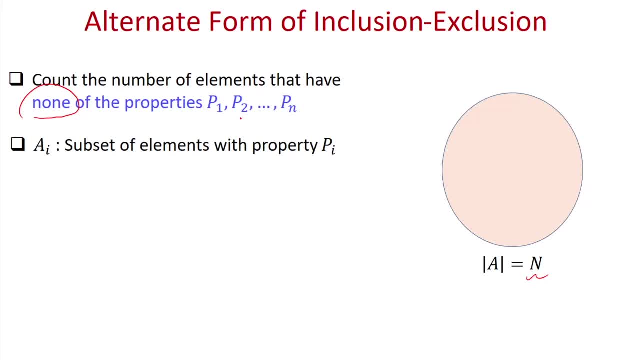 So for that, what we will do is we will first identify the subset A i consisting of elements which has property p i. I stress, A i is the set of elements in the set A Which has the property p i. And if I take the union of the subsets A1 to A? n, I get all the elements in the set A which has either the property p1 or the property p2 or the property p3, or so on. 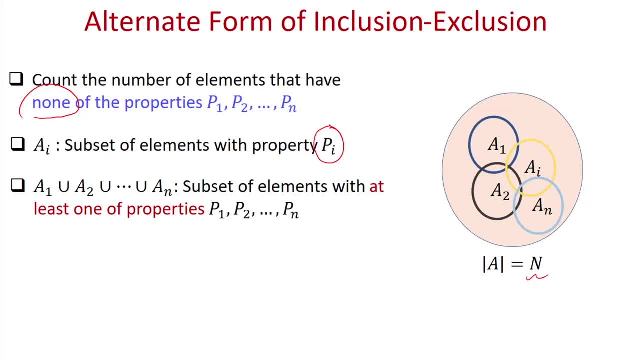 That means it will have at least one of the properties p1 to pn. But that's not what we want. We are interested in the elements which do not have any of these properties. So it's easy to see that now the desired answer, or the number of elements which do not have any of the properties p1 to pn, will be the difference of the cardinality of A, which is n, and the cardinality of the union, of n sets. 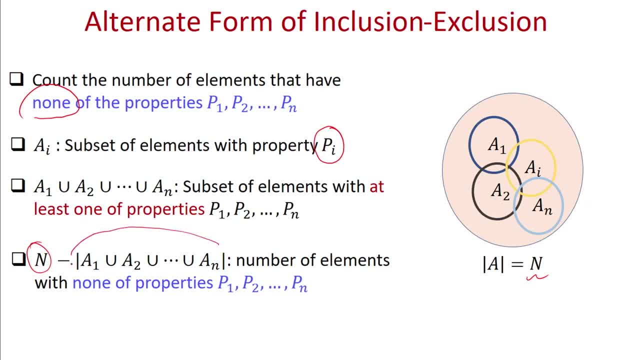 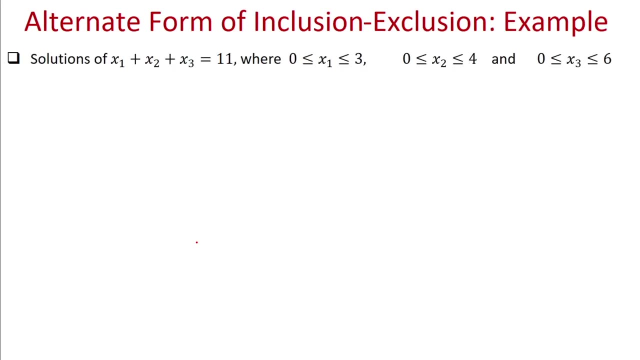 And now we will apply the rule of inclusion-exclusion to find out the cardinality of the union of the n sets, because we know how to find that. So this is the alternate form of inclusion. So let me demonstrate this alternate form of inclusion-exclusion through some examples. 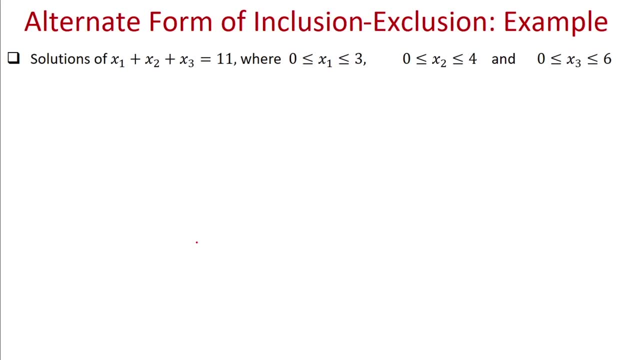 Suppose we want to find out the number of solutions for this equation- number of integer solutions- And my restrictions are: x1 should be in the range 0 to 3, x2 should be in the range 0 to 4 and x3 should be in the range 0 to 6.. 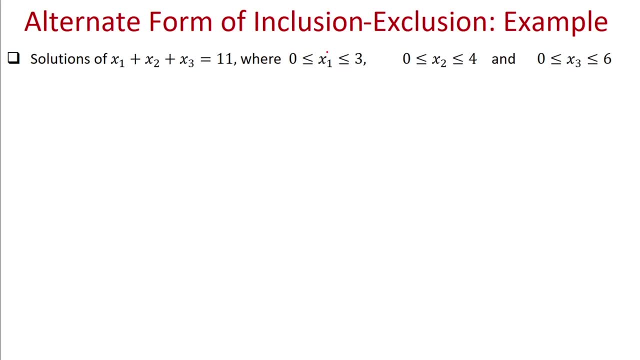 Now using the methods that we have seen till now. we can't find it directly, But what we will do is the following: We will use the alternate form of inclusion-exclusion, So we will first find out the cardinality of the universal set. 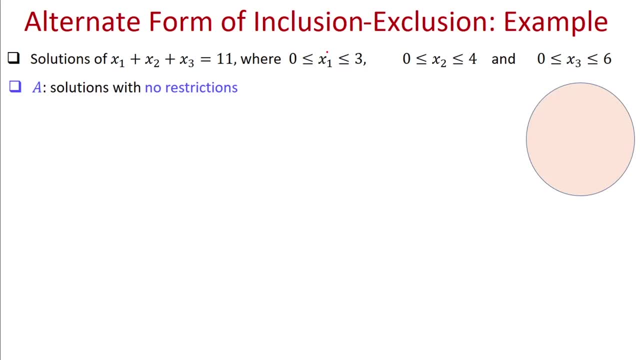 Universal set in this context will be the set of all solutions where I don't put any restrictions on x1, x2, x3. So they could be anything. In fact, I can have a solution where x1 is 11 as well. 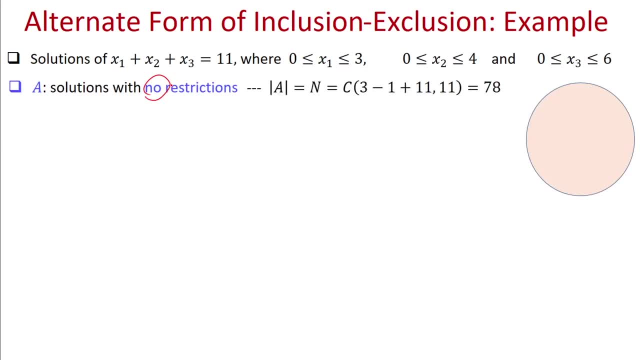 And I know the cardinality of this universal set Because that comes from the formula for combinatorics with repetition. So it's equivalent to saying that we have to select 11 bills And we are given bills of either denominations x1, x2 and x3. 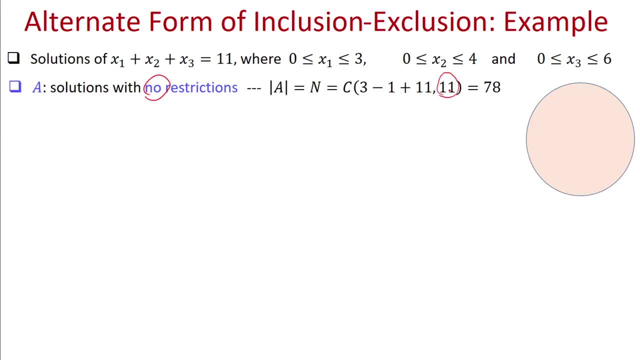 And I have no restriction, Because that's what is the interpretation of the set A. Now let me define a set A1 to be the set of solutions for this equation where x1 is greater than 3.. So now you see your property P1 was that your solution should not have x1 more than 3.. 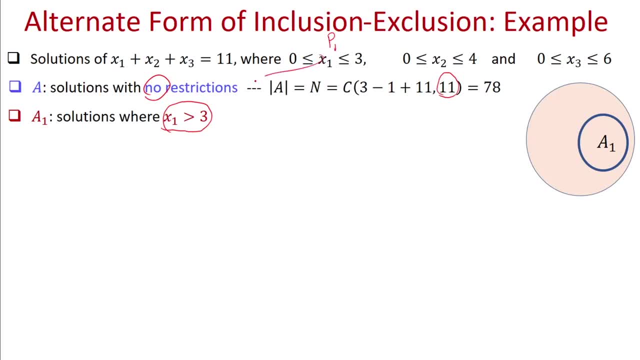 But I am now finding solutions which violate the property P1. Namely, solutions where x1 is allowed to be more than 3. In fact, x1 has to be more than 3. And we know how to find the cardinality of A1 set. 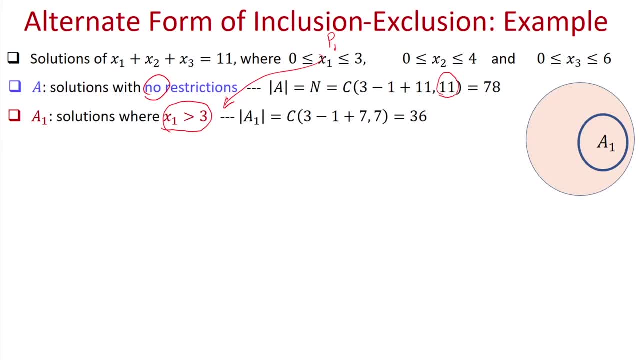 If x1 is more than 3. That means I have to definitely pick 4 bills of x1 type. So I will be left with now selecting 7 more bills without any restriction, And the number of ways of doing that is 36.. 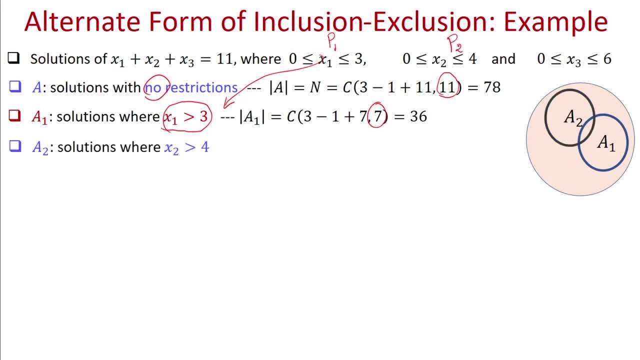 In the same way, my property P2 is that my solution x2 should be strictly less than equal to 4.. But now I try to find out solutions which violate the property P2. Namely solutions where x2 is definitely greater than 4.. 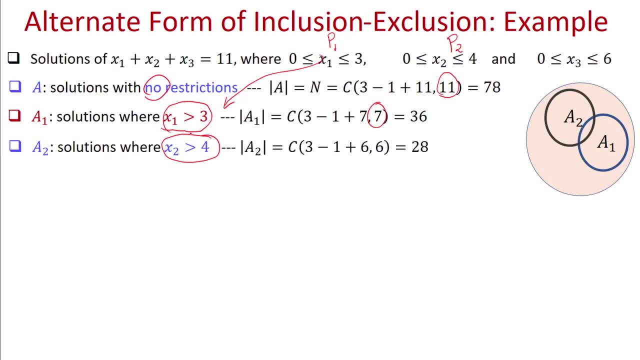 And let A2 be the set of such solutions. The cardinality of A2 will be this, And similarly my property, P3, could be that I am interested in solutions where x3 should be less than equal to 6. But then I try to find out solutions which violate this property. 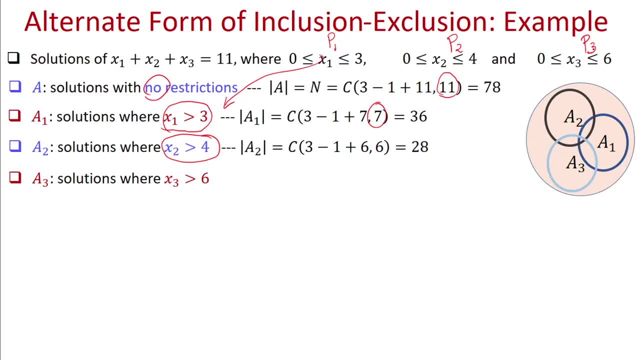 And define the set of such solutions to be A3.. And the cardinality of the set A3 will be this. And now it's easy to see that my overall solution, The number of overall solutions, will be The difference of the cardinality of the universal set, which is 78.. 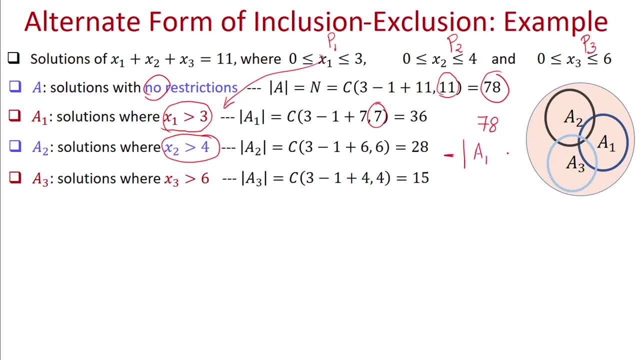 And the cardinality of the union of the set A1, A2 and A3.. Now to find out the cardinality of the sets A1, A2 and A3. I have to use the principle of rule of inclusion- exclusion. For that I need the cardinality of pairwise intersection of sets. 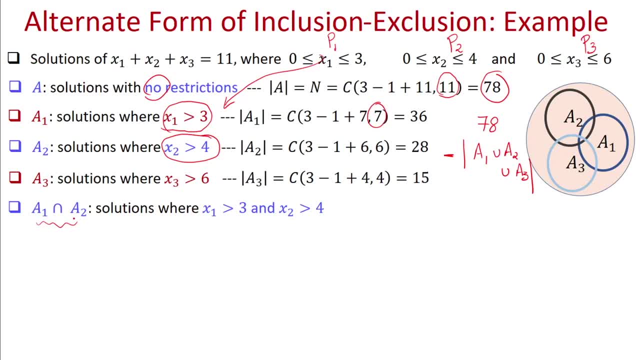 So let's find out the cardinality of the set A1 intersection A2.. So A1 intersection A2 means the solutions where both x1 is greater than 3 as well as x2 is greater than 4.. And it's easy to see that the number of solutions 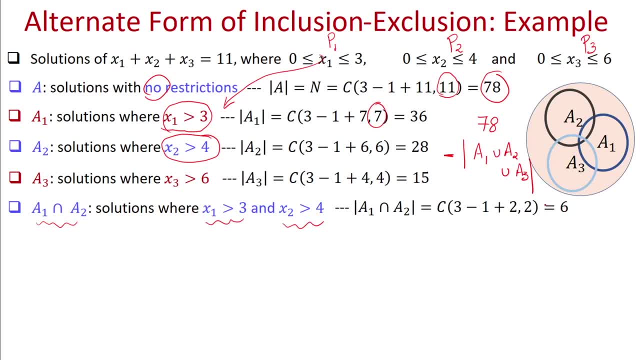 The number of solutions of such type will be this, Because if x1 is greater than 3, that means x1 is at least 4.. That means I have picked 4 bills of type x1. And if x2 is greater than 4, that means x2 is at least 5.. 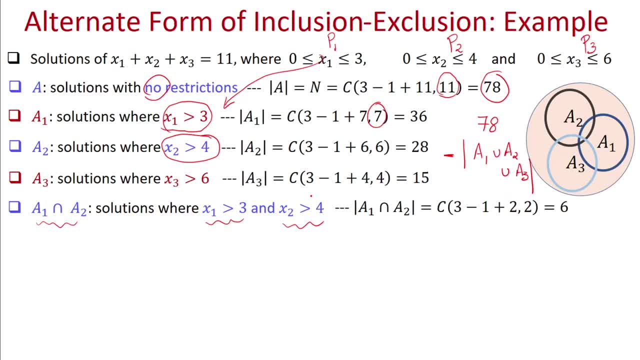 That means I have picked 5 bills of type x2.. So that means overall 9 bills have been already picked, And I am now left with the problem of choosing 2 bills of either denominations x1,, x2, x3, without any restriction. 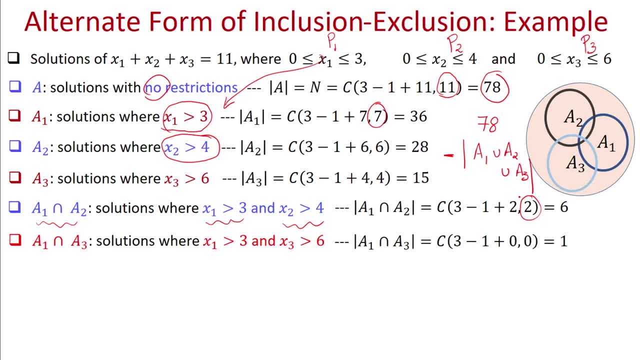 Similarly, the cardinality of A1 intersection A3 will be this: This is because if x1 is greater than 3, that means x1 is at least 4.. And x3 greater than 6 means x3 is greater than equal to 7.. 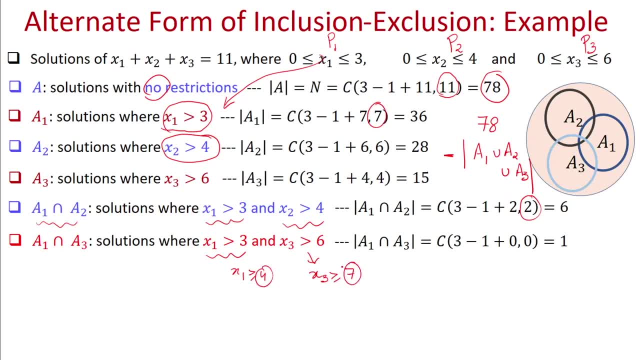 That means I have already chosen 11 bills. That means there is only one solution possible where x1 is greater than 3 and x3 is greater than 6.. Similarly, take x1 to be 4 and x3 to be 7.. 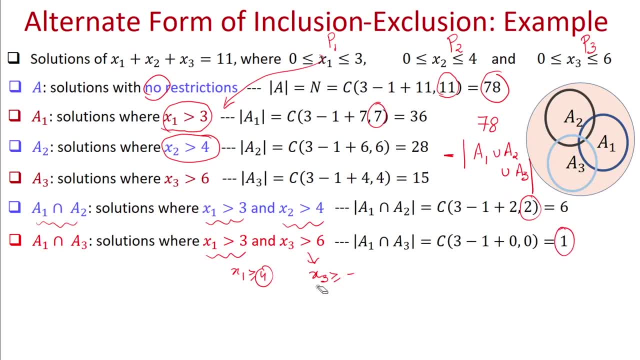 That's why the number of solutions or the cardinality of A1 intersection A3 is 1.. Similarly, if I take A2 intersection A3, it turns out that there are no solutions, Because I can't have any solutions where x2 is greater than 4 and x3 is greater than 6.. 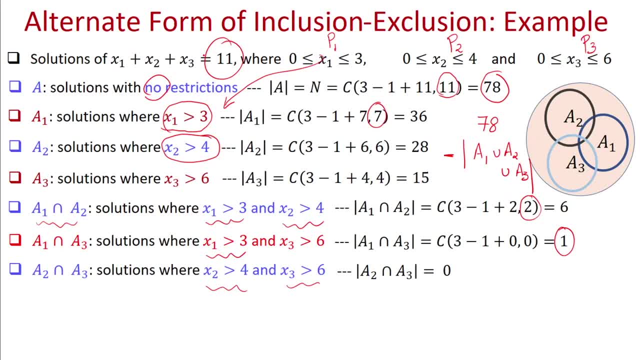 Because overall, the sum of x1, x2, x3 should be 11. If I take the intersection of A1, A2.. Again, there are no solutions. And now I have all the things to find out, the cardinality of union of A1, A2, A3. 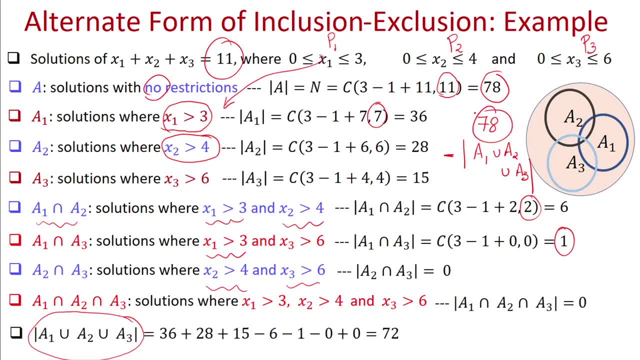 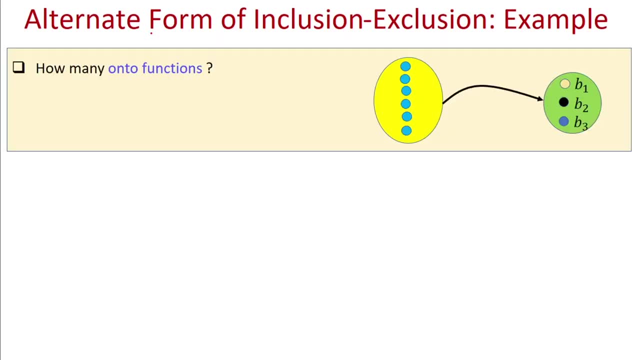 And, as I said, if I subtract it from my universal set cardinality, then that will give me the number of required solutions. So now you can see that how I use the alternate form of inclusion exclusion for solving this problem. Let's use alternate form of inclusion exclusion. 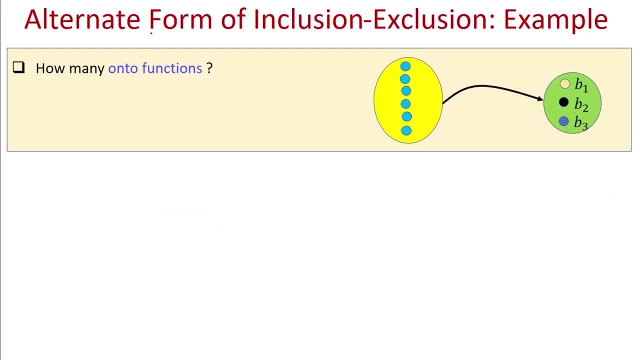 To solve another problem. So you are given two sets A, set A consisting of six elements And another set B consisting of three elements, And I am interested to find out how many onto functions are there. Well, we already have found the answer for this in one of our earlier exercises. 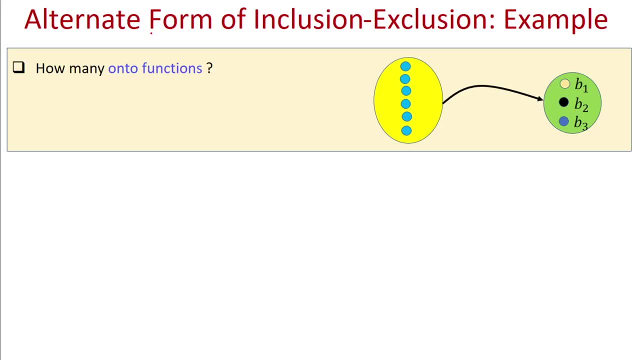 Using sterling numbers of second type, But now I will be using the alternate form of inclusion exclusion to solve this problem. So, for finding this and using the alternate form of inclusion exclusion, What we will do is We will find out the total number of functions. 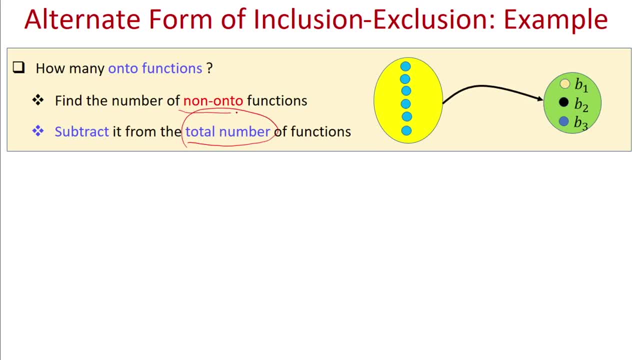 And from that we will subtract the total number of non onto functions. So let's define the set A to be the set of all functions And it is easy to see that the cardinality of the set A is 3, power 6.. Because I have six elements. 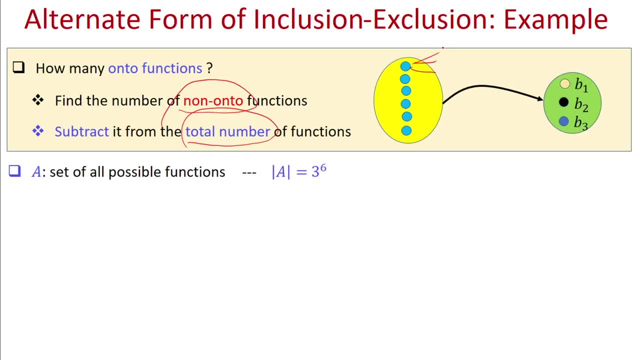 For each of the elements, I have three possible images to pick from Mind it. the set A has all the functions which are onto As well as all the functions which are non onto. Now I will be subtracting the number of non onto functions. 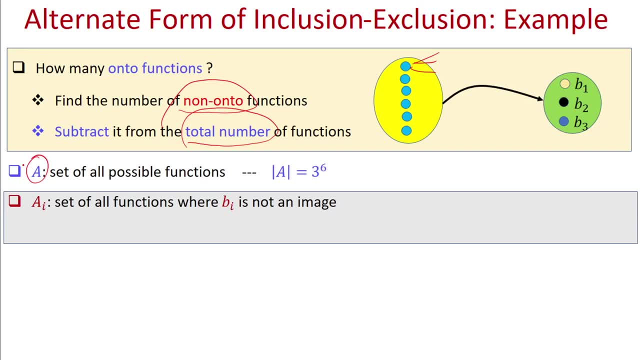 For that I define a subset A i to be the set of all functions Where the element B, i is not an image. Okay, So it is like saying the following: An onto function will have the property that B1 has an image, B2 also. 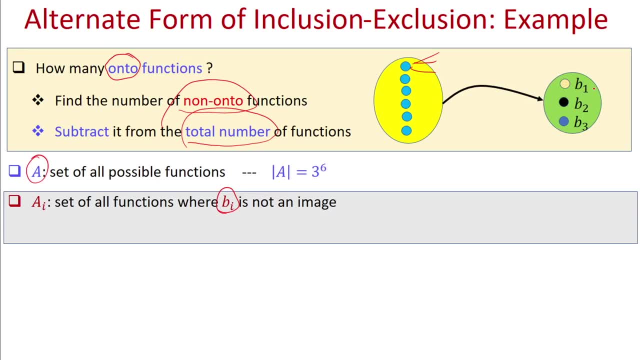 B1 has a preimage, B2 has a preimage, As well as B3 has a preimage. Okay, So these are my three properties. If any of these three properties is violated, I get a non onto functions. So that's what I am now trying to find out. 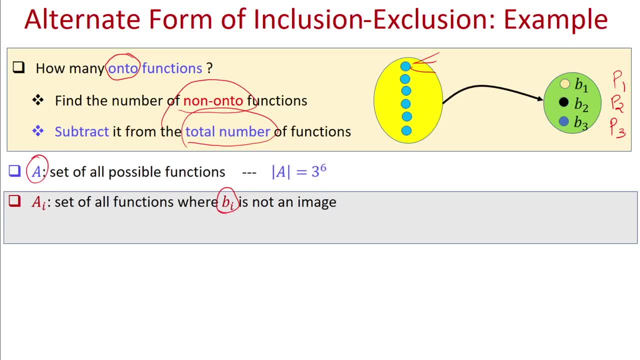 How many ways I can violate these properties To B3.. So I try to analyze how many ways I can violate the property P i. So property P i is the element B, i is an image, Whenever I am picking a function. So violation of that property will be. 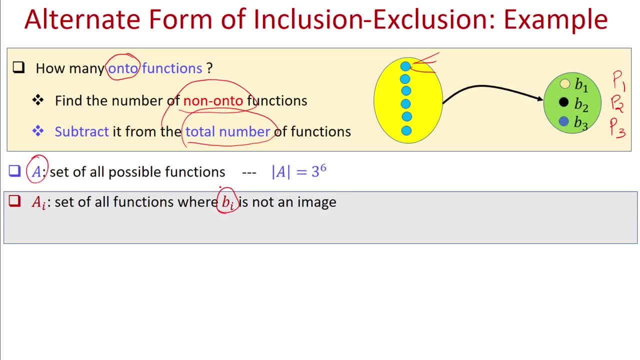 That element B i is not chosen as an image When a function is Formed from the A set to the B set, And let A of i denote The set of all such functions Where the element B- i do not have any preimage. 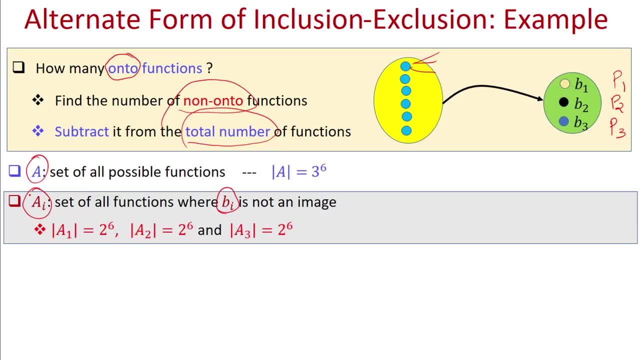 Okay, So for instance, The set, The cardinality of the set, A1 will be 2 power 6.. Because if B1 is not allowed to be a possible image, Then for each of the six elements I have two possible images to assign. 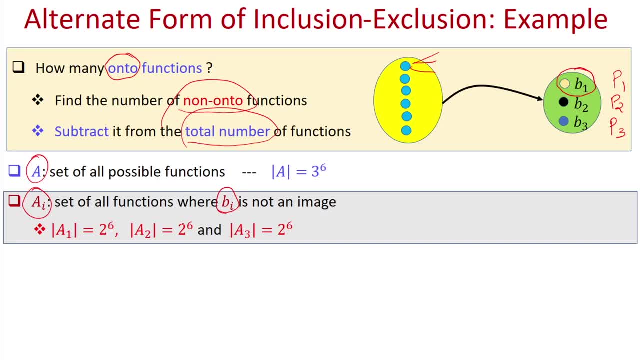 Either B2 or B3.. In the same way, the cardinality of A2 also will be 2 power 6.. Because A2 means the element B2 is not allowed to be a possible image, That means the only images could be B1 or B3. 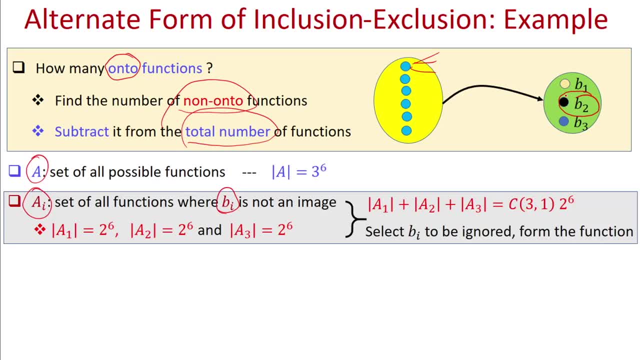 And so on. So I can say that If I take the cardinality of Add, if I take the, If I add the cardinalities of A1,, A2, A3. Then that is same as the following: You first select the element B, i. 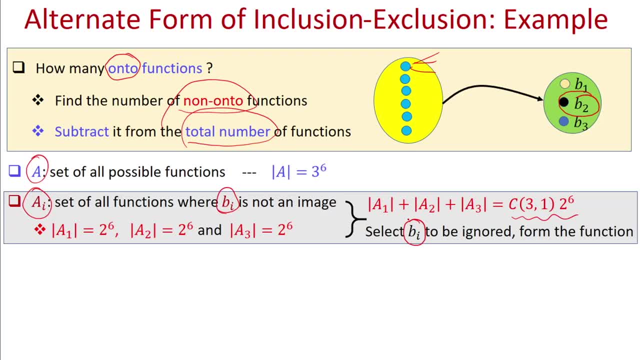 Which should be ignored, That means Which should not have a preimage And then form the function From the A set to the B set With respect to the remaining two elements, So the element B i, Which has to be ignored. 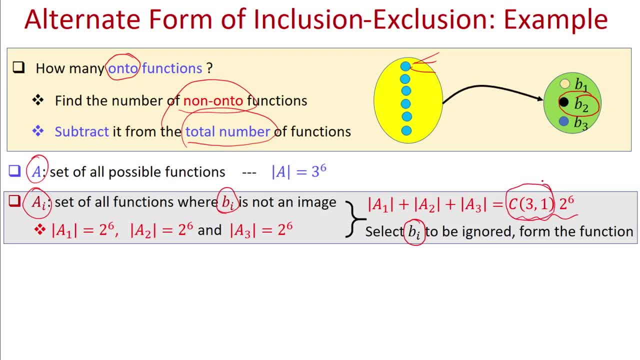 It can be chosen in three. choose one ways And now you are left with only two elements. So each of the elements in the A set Can be assigned those two images. So this will be the overall count If I take the Summation of the cardinalities of the sets A1,, A2, A3. 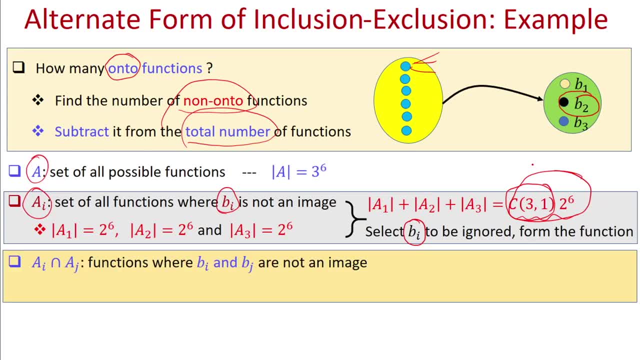 Now, if I take the Pairwise intersections of A- i and A- j sets, Then basically They denotes the functions Where neither the element B i nor the element B j Can be the possible images Right. So for instance, The cardinality of the set A1, intersection A2.. 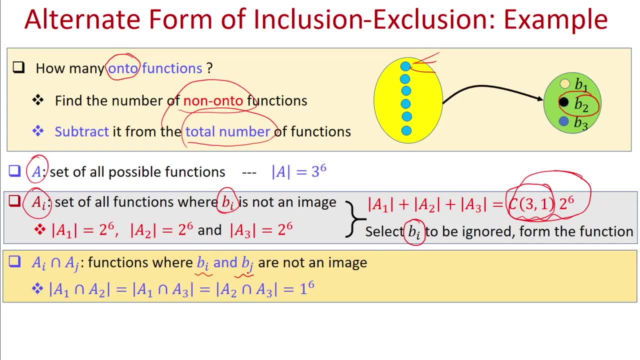 Where we want power: 6. Because A1 intersection A2 means the following: You can't have element B1 as a possible image. You can't have the element B2 have a possible image. That means We are considering the function. 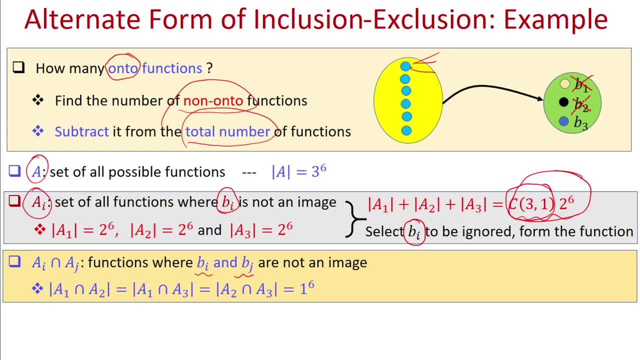 Where all the elements are mapped to B3. So there is only one power six. such functions, Basically one Same way. The cardinality of A1, intersection A3. Will be one power six, and so on. So again We can say that. 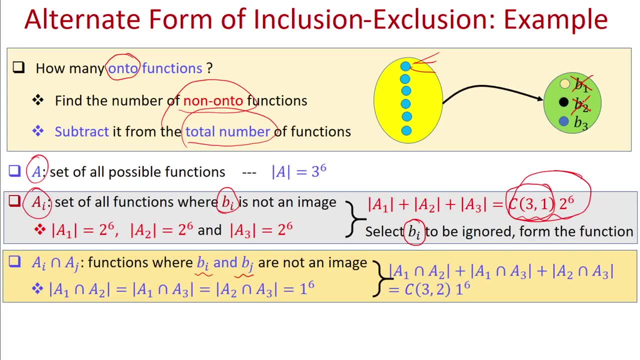 If we take the summation of the cardinality Of the pairwise intersection of sets, Then that will be same as the following: You find out the two elements Which have to be ignored, That means Which are not allowed To be the possible images. 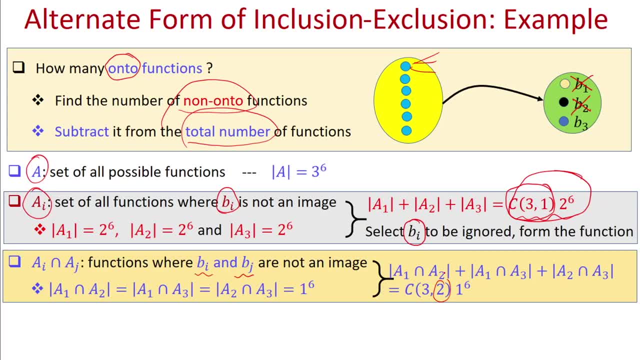 So you can do that in Three, choose two ways, And then you will be left with only one element, Which is the only allowed image, And then if I take the cardinality of Intersection of three sets at a time, Then the interpretation of that will be: 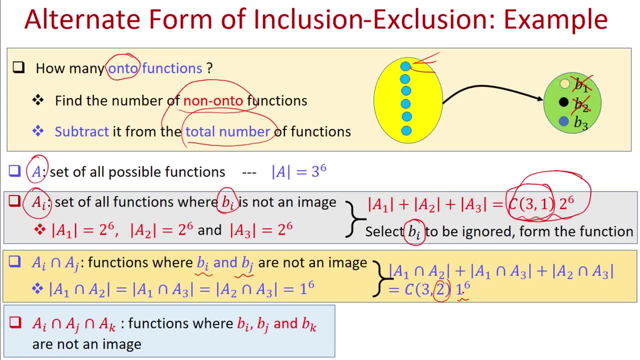 I am considering functions Where neither the element Bi, Bj and Bk Are allowed to be possible images. Well, in this example, Since I have only three possible images To choose from, I am saying that I want to design a function. 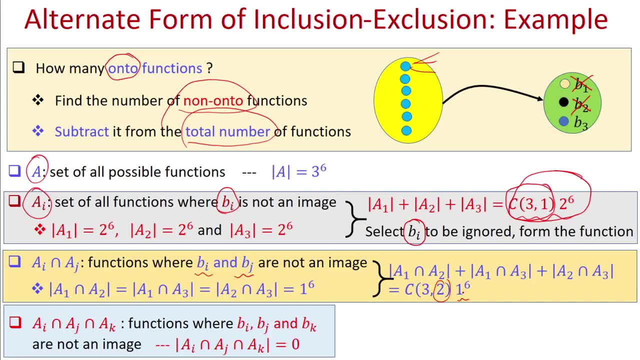 Where none of those three elements Can be the images, And I can't have any such function. So that's why The cardinality of the Intersection of triplets of set Will be zero in this case. So, as I said now, 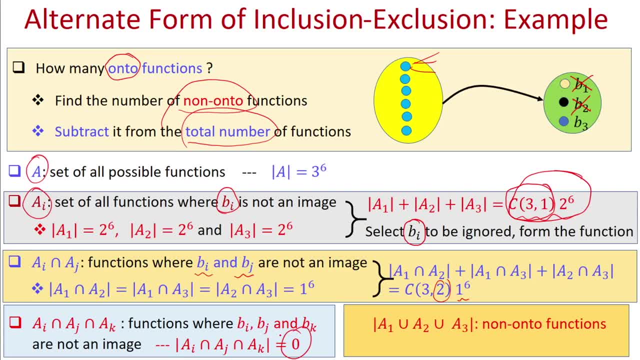 The union of A1, A2, A3. Will give you all the non onto functions, Because the union of these three sets Will have those functions Where either B1 is not allowed To be an image Or B2 is not allowed to be an image. 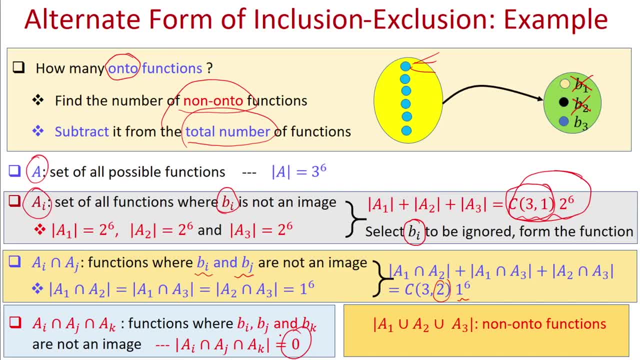 Or B3, is not allowed to be an image. Okay, And As per the rule of inclusion exclusion, The number of non onto functions Will be this: And if you subtract this quantity From this value, The size of the universal set. 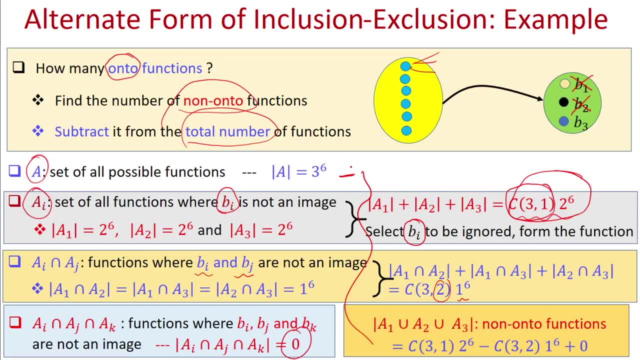 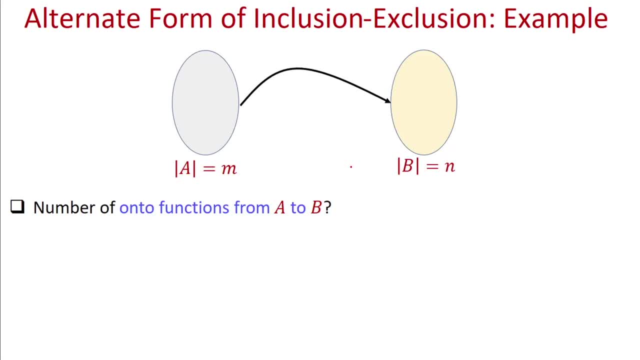 That will give you the Number of onto functions. Okay, So now let's generalize this formula. So in the previous case we took, We had the case where A was 6. The cardinality of Where the set A: Okay, 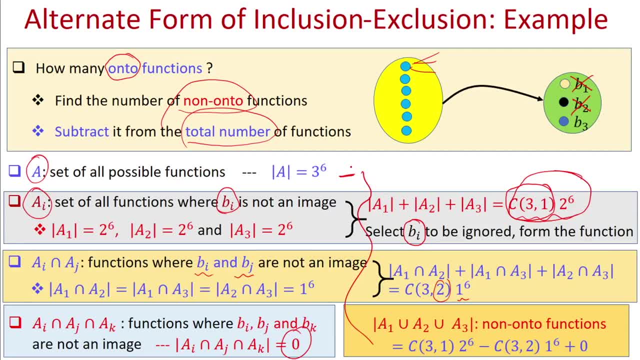 Where the First set has 6 elements And the set Of possible images has 3 elements. Namely, my M was 6. And my N was 3. So now We want to generalize it. We have a set A. 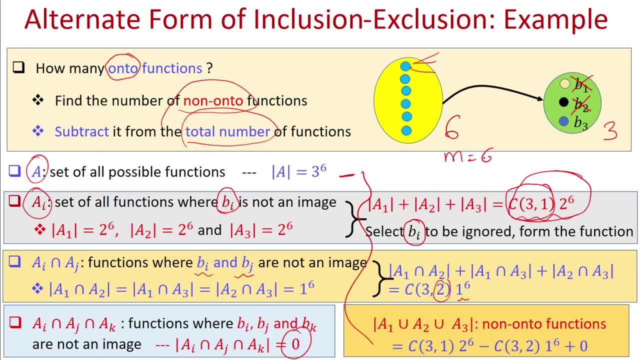 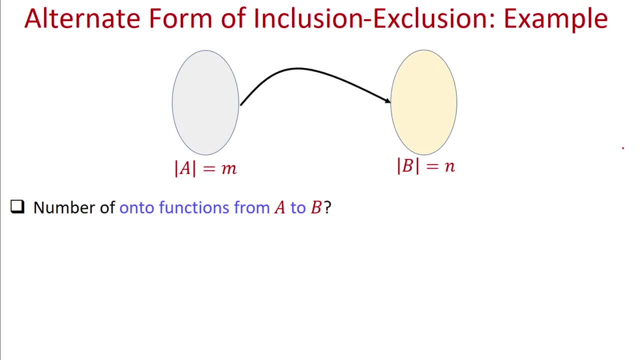 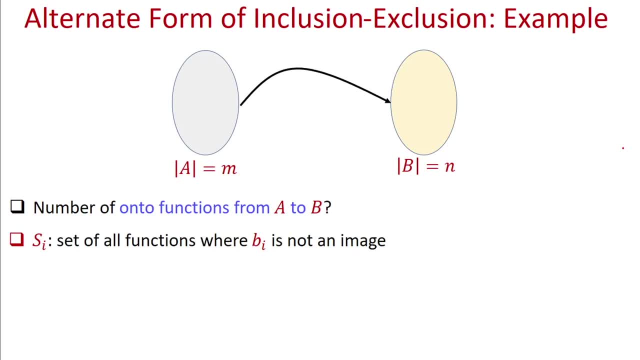 I just, I just I mean my burns B Enough to be a B Sue for A. set B Is equal to A. set B Is equal to N. elements S All Some doesn't apply To. 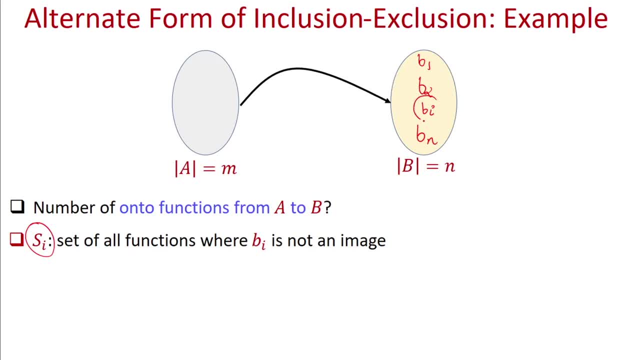 The position of the set B, That So Our, That Part Of conjunto, Zeta X, Y And Seta. So the Entropy Peshelf is 0. At all. We basically 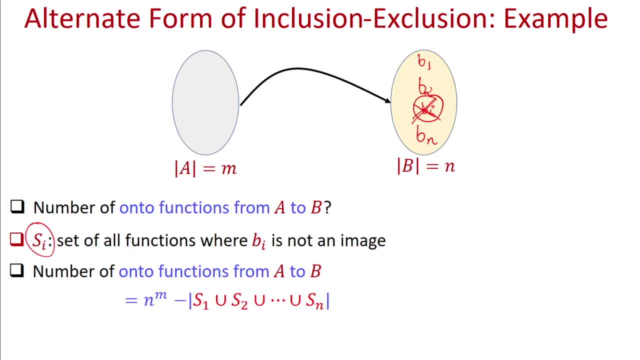 Are, As we did in the demonstration in the earlier slide. the total number of onto functions will be the difference of the number of all possible functions, which include both onto and non-onto functions, and the number of non-onto functions. And the number of non-onto functions is given by the cardinality of union of the sets S1. 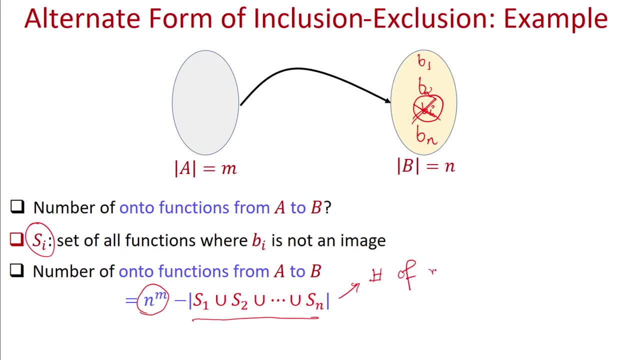 to S7.. So this is the number of non-onto functions And if we expand this cardinality of the union of S1 to SN, then it will turn out to be this right. So the first term here denotes basically that the cardinality of S1 plus S2 plus S of 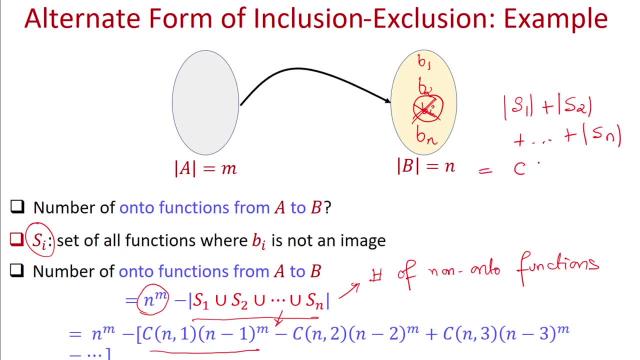 N is nothing, But you decide the single element which is not allowed to be image. That can be done in N. choose one ways And then the remaining N minus 1 elements in the set B could be the images for the elements in the set A. 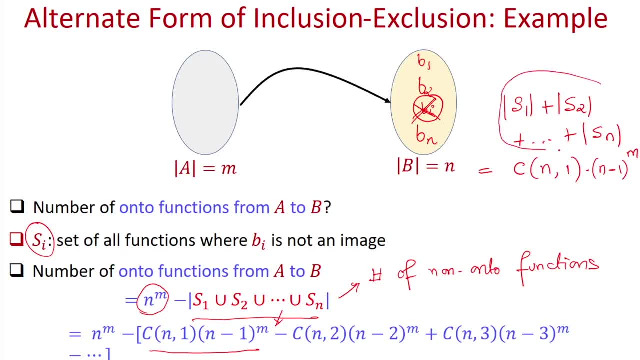 So overall contribution of the cardinality of S1 to SN will be this: Similarly, if I want to take the pairwise intersection and their cardinality cardinalities and sum them up, then it is equivalent to saying that SI intersection, SJ basically denotes all those functions where neither BI nor BJ can be the images. 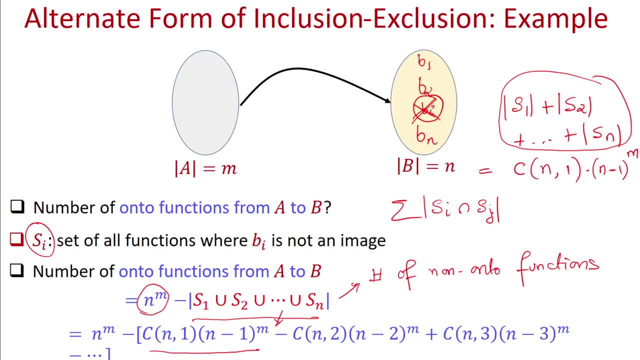 That means the remaining n minus 2 elements can be the images. Now this INJ can be any INJ, from the set 1 to n, okay, the indexes. So that's why it's equivalent to saying that you decide, you choose the two elements, I and J, or BI or BJ, which are not allowed to be. 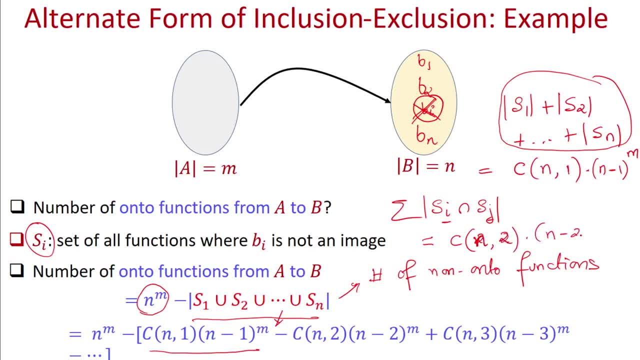 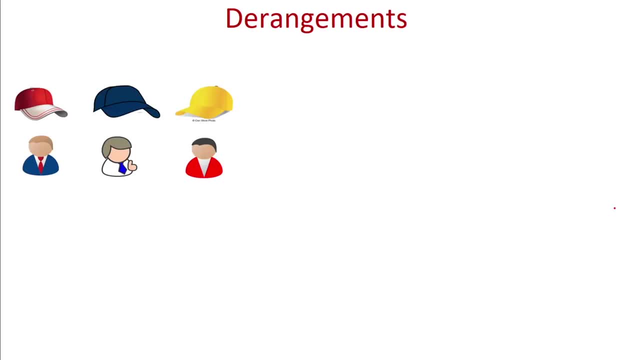 the images, and then your function will have the remaining n minus 2 elements as the possible images. okay, and so on. Right Now, our last case study for alternate form of inclusion-exclusion is the number of derangements. So what exactly is a derangement? So imagine: 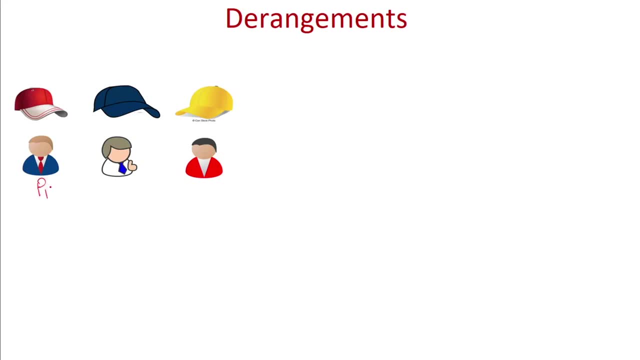 you have three people, three person person one, person two and person three, and they have their respective caps, caps, cap one, cap two and cap three. Now a derangement caps. derangement of the caps is an arrangement of the three caps. 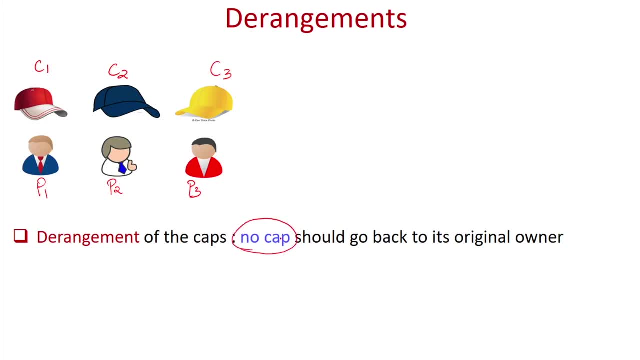 so that no cap go back to its original owner. So this is one of the derangements. right Now, person one gets the cap number C3,, person 2 gets cap number C1, and person 3 gets cap number C2,. okay, 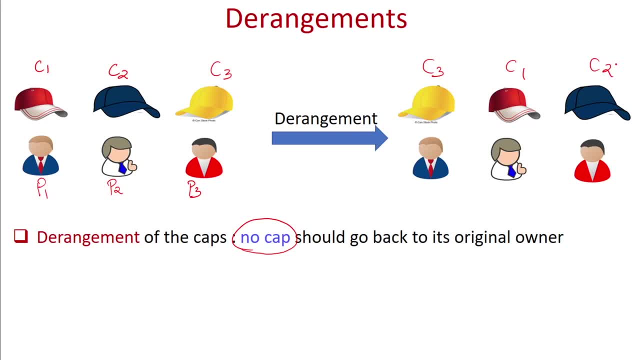 So none of the person gets, or the original owner gets back, none of the person gets back its original cap. So that's an derangement, okay, And derangement of n objects basically denotes a permutation of those objects such that it: 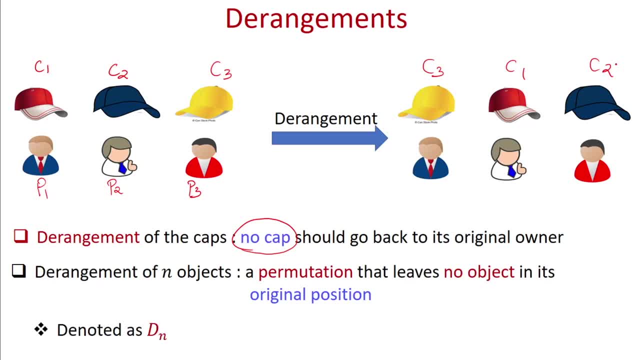 leaves no object in its original position, and number of derangements of n objects is denoted by this quantity d of n. okay, So d of 1 is 0, because if there is only one object and you can't derange it, it will. 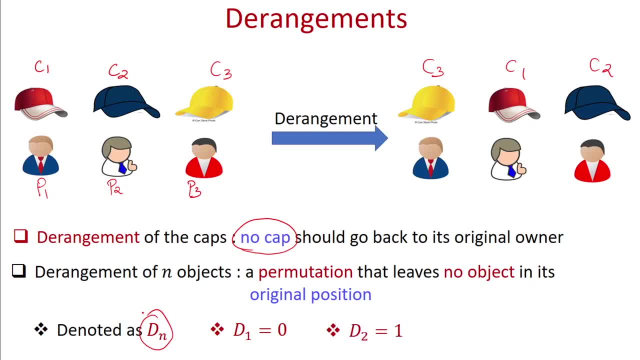 be at its position And d of 2 is 1, because if you have cap number 1 at position 1 and cap number 2 at position 1, then the only way to derange it is derangement: Take cap number 1 to position 2, and take cap number 2 to position 1, and so on. okay, 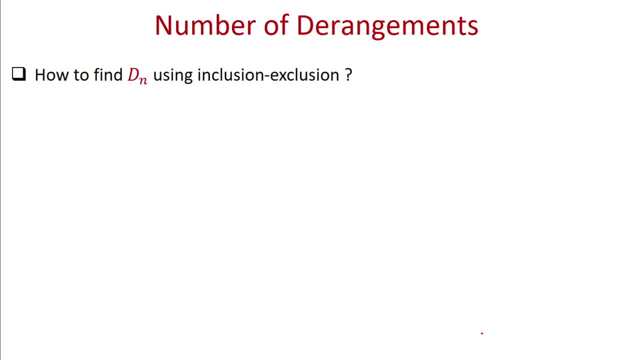 So we want to find out the number of derangements, namely the value of d of n, And there are several ways of doing that. In the tutorial we will derive a recurrence relation. In this lecture we will see how to find out the value of d of n using the alternate form. 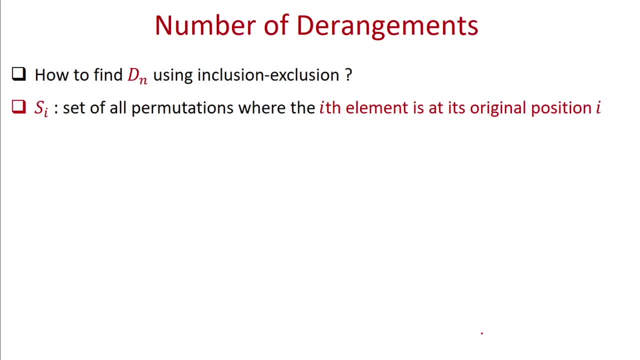 of inclusion-exclusion. okay. So again, remember, in the alternate form of inclusion-exclusion, you have to identify the property P And then you have to see how, in how many ways, you can violate the property P. Okay, So, property P. 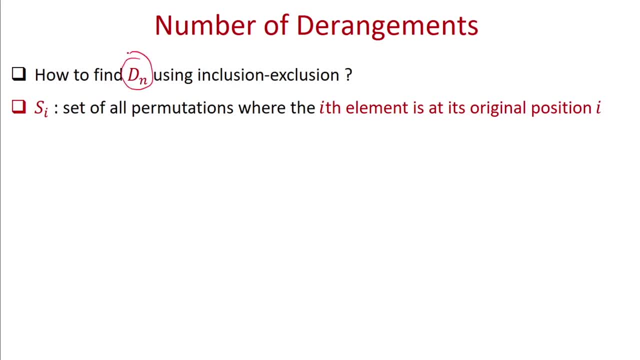 With respect to the derangement is that you do not want the ith element to be at the position i, because if ith element is still there at position i, then that's not a derangement. We want to violate that property, So let S of i denote the set of: 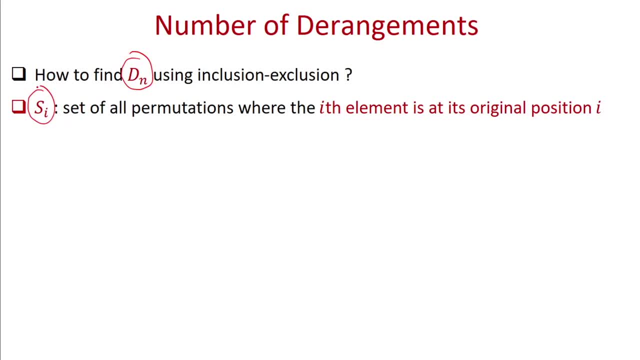 All possible permutations of n elements. okay, where the ith element is still at its position, namely it is still at the position i. okay, So it's easy to see that the cardinality of the set S i is n minus 1 factorial, because 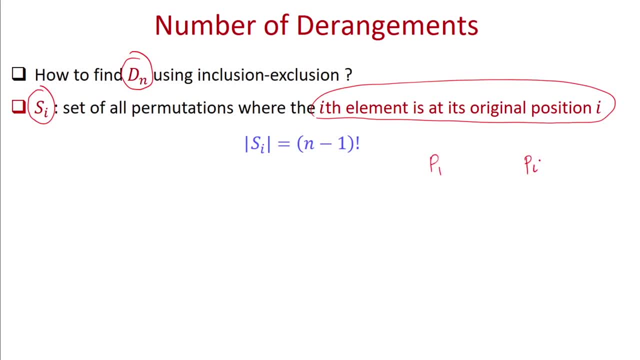 think of it as follows: You have position 1, position i, position n. You are finding all possible, All possible permutations where the element i is definitely at its position, namely i. it's still at position i. I don't know what is the status of the remaining n minus 1 values. 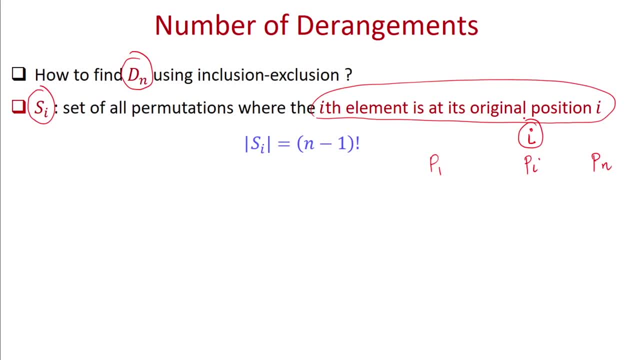 They may be at their position, some of them may be at their position, none of them may be there at their position, and so on. So it's equivalent to saying that I am interested to permute the remaining n minus 1 elements. 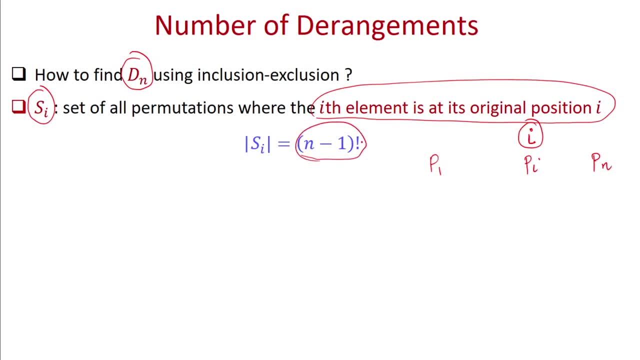 which can be done in n minus 1 factorial ways. So that's the cardinality of Okay, The set S, i and, as per our definition, if I take the union of sets S 1 to S n, it gives me all the permutations where at least one of the elements is still at its original position. 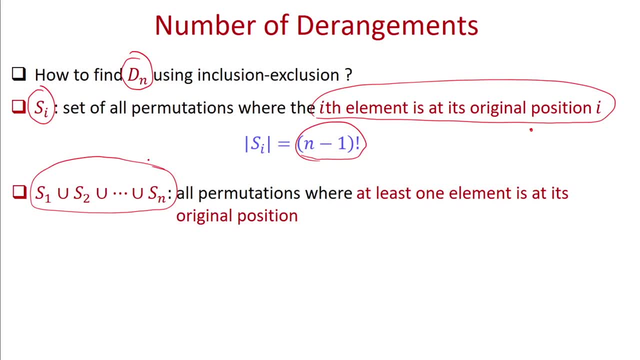 It could be either the first element or the second element, or the third element or the nth element. That means the arrangements or the permutations. in the union of the sets S 1 to S n are the permutations, Not the derangements. 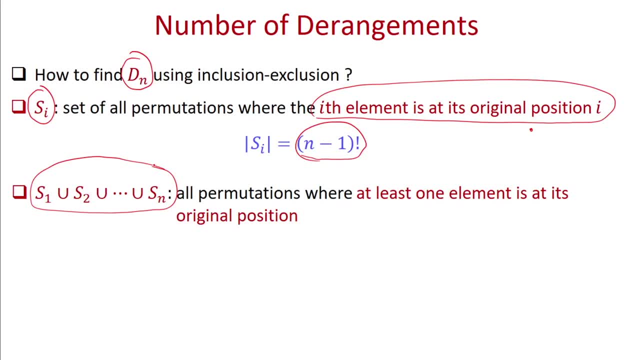 Because, as per derangements, as per a derangement, none of the n elements should be at its position. So that means, as per the alternate form of inclusion, exclusion, the value of D of n will be the cardinality of the universal set. 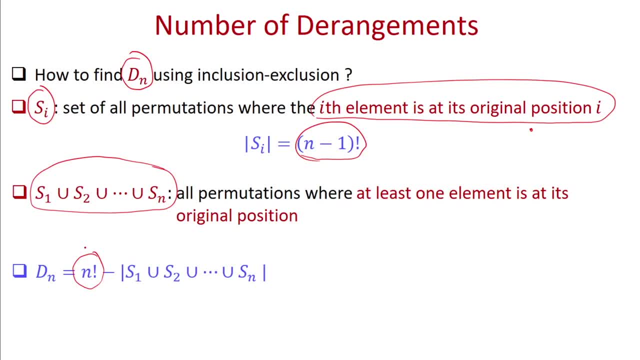 The universal set in this case will be the set, the number of all possible arrangements or permutations of n elements. They could be derangement or they may not be derangements, So this is n factorial. Okay, From that I have to subtract the cardinality of the union of the n sets. 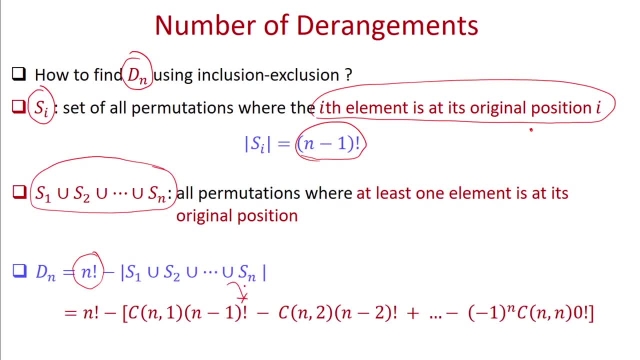 Now, if I expand the cardinality of the union of n sets, it will turn out to be this: So, if I take the effect of the summations of all S, i's the cardinality of the summations of S i. this will be same as you pick the element i, which is still at its position. 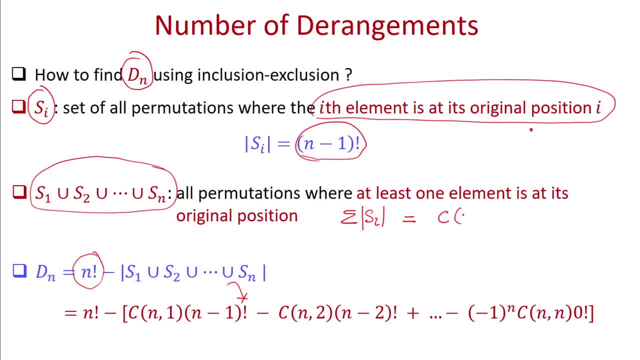 namely at position i. That could be done in n choose 1 ways. And then the cardinality of each set S i is n minus 1 factorial. Similarly, if I take the cardinality of intersection of S i and S j, then the elements i and j 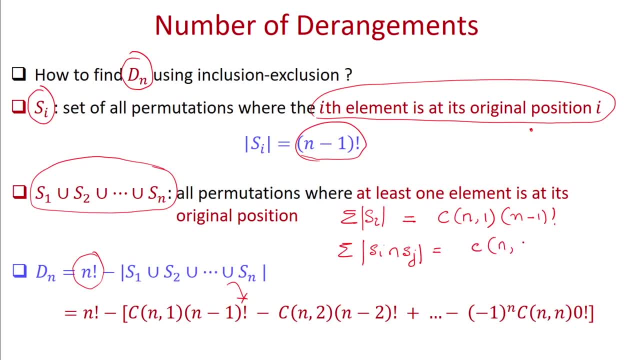 can be chosen in n choose 2 ways. That means S i, intersection S. j denotes all those permutations where the ith element is at position i And the jth element is t, So it is still at position j. That means the remaining n minus 2 elements can be permuted in any order, and so on. 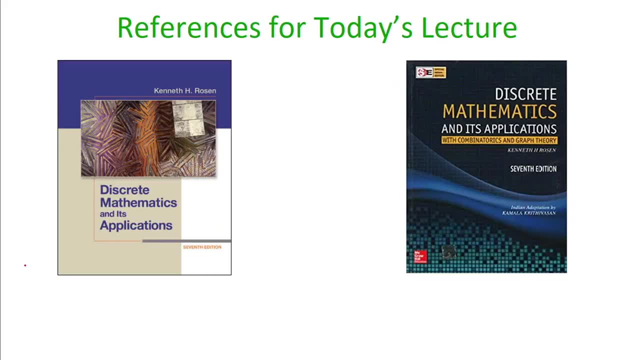 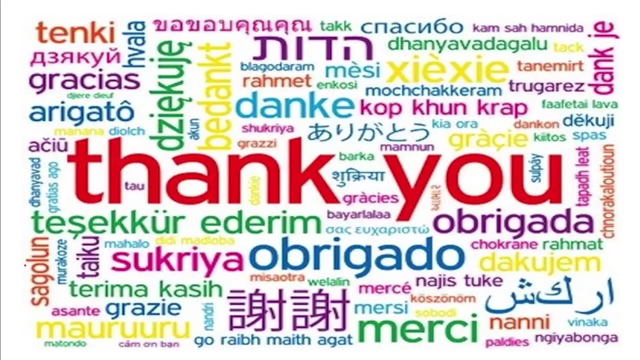 So that will give you the value of d of n. So these are the references for today's lecture, And with that I end this lecture. Just to summarize: in this lecture we discussed the principle of inclusion-exclusion. We derived a formula for that. 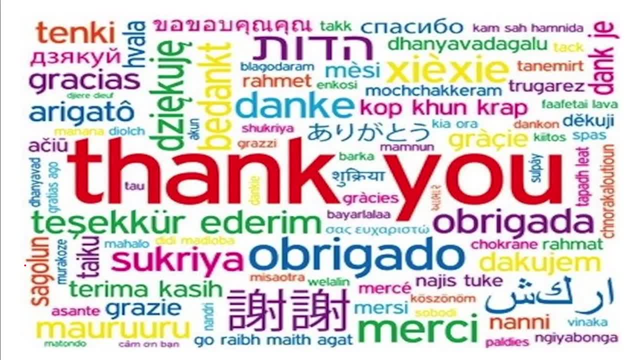 And we saw an alternate form of inclusion-exclusion. Okay, And some case studies for the alternate form of inclusion and exclusion. Thank you,